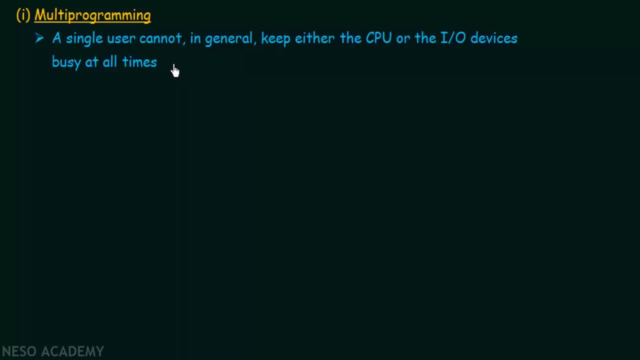 because it is not capable of multi-programming. But in multi-programming, what will happen is that it increases the CPU utilization by organizing the jobs, which are codes and data, so that the CPU always has one to execute. So that means that in multi-programming, 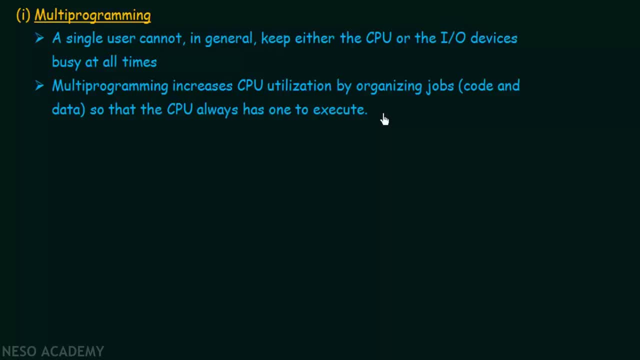 what we are trying to do is we are trying to increase our CPU utilization, because the CPU is capable of executing multiple programs. So let's see how this works. So in this diagram we have the job pool and the memory layout of the multi-programming system. 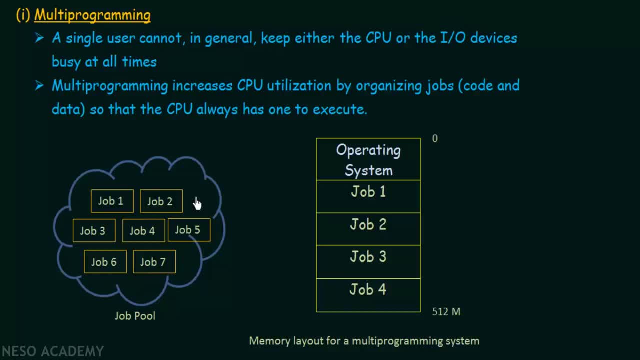 So first of all, let us understand what is a job. So, job is something that has to be executed, which may contain codes and data. So here we have a job pool which consists of all the jobs that enter the system, So all the jobs that has to be executed. 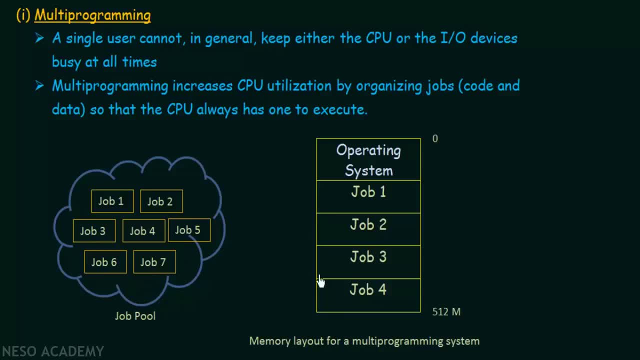 they are kept in a job pool like this. And then here we have the memory layout of a multi-programming system. So on top we have the operating systems and these are the jobs that are loaded into the memory. So we cannot load all the jobs that are loaded into the memory. 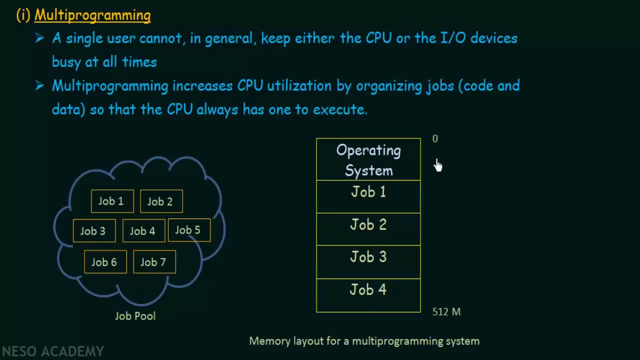 So all the jobs in the job pool into the memory, because we don't have unlimited memory or memory is limited. So by memory I mean the main memory or your RAM. So here in this example we are having 512 MB of RAM over here. 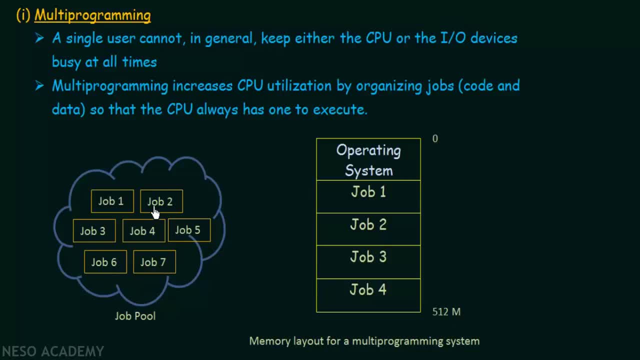 So you are not able to load all of this into the main memory. So a subset of these jobs or some of these jobs are loaded into the memory. So for this example, we have loaded job 1,, 2,, 3 and 4 into the memory. 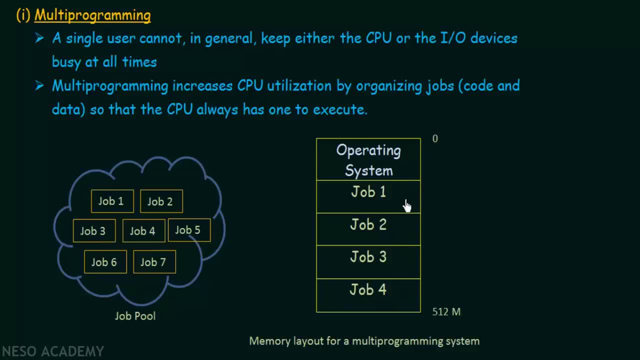 Now this operating system has to help in executing these jobs by assigning the CPU to these particular jobs. So if we don't have this multi-programming, what will happen is that job 1,, let's say, starts executing and is using the CPU. 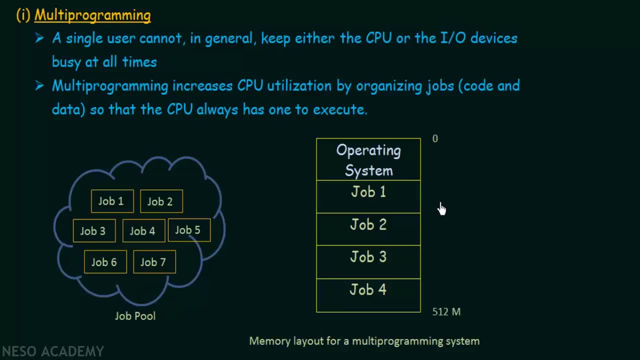 Now, until and unless job 1 finishes its execution completely, the other jobs cannot use the CPU. So let's say that job 1 was using the CPU and then it has to use some other resources in the core surface execution, Let's say the I O devices. 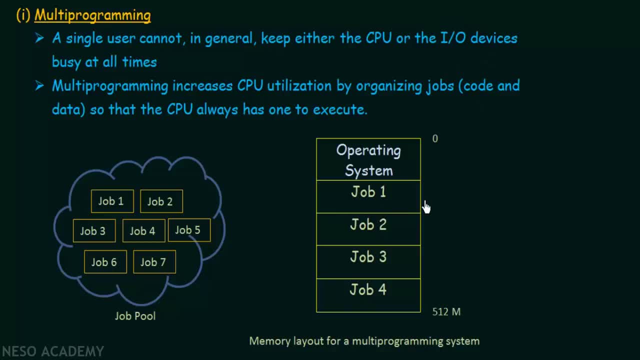 Now, when job 1 goes to use the I O devices, the CPU is not used and the CPU just stays idle without being used by any other jobs. So that is a very inefficient way. So in multi-programming what happens is that: 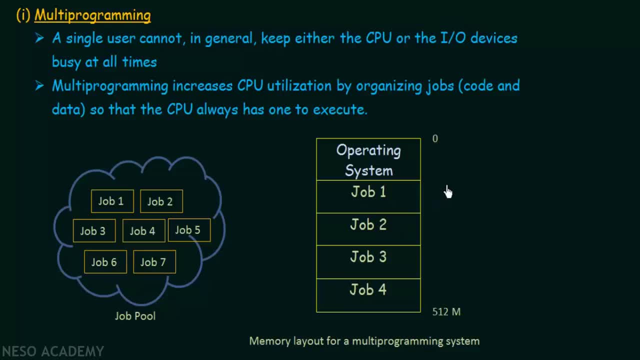 let's take the same example again. job 1 starts executing and is using the CPU and on the course of its execution, job 1 tries to use the I O devices. So when it goes for using the I O devices or any other resources, 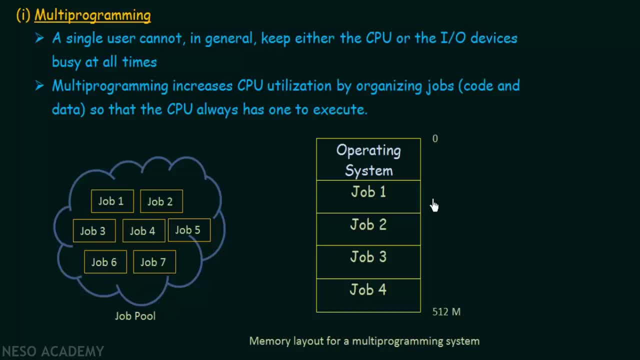 the CPU is released by job 1.. And then that CPU, instead of remaining idle, it can be used by another job, let's say job 2. So job 2 can use the CPU until job 1 finishes its other I O device operation. 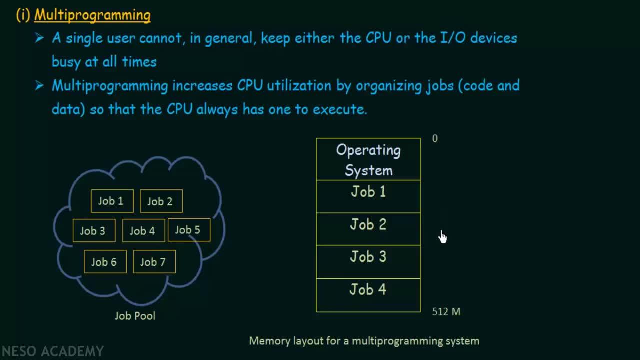 and wants the CPU back. So job 2 will be using the CPU. and again, if let's say job 2 wants to go for using some other resources and does not need the CPU at a particular time, then the CPU again instead of remaining idle. 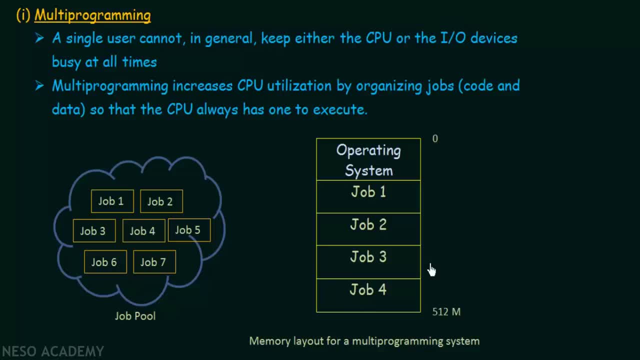 can be used by job 3 and so on. So in this thing we see that the CPU does not remain idle. Whenever a particular job does not want to use the CPU, the CPU can be utilized by another job. So this is a very efficient system. 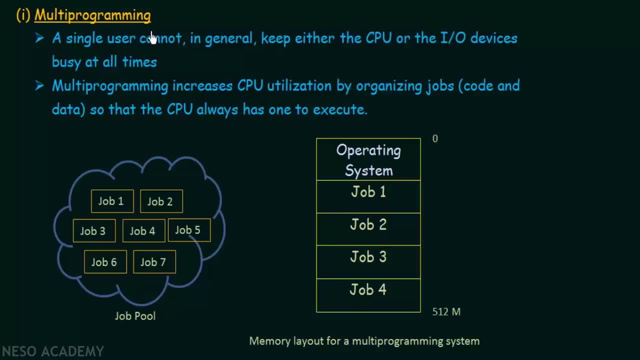 or an efficient way of executing. So that is what multi-programming is mainly about. So we see that for operating system to be efficient, it should be capable of this multi-programming. So we can also relate this multi-programming with our day to day life. 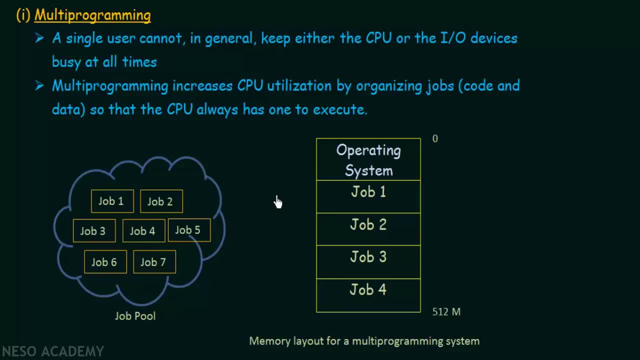 So let's say that, for example, there is a lawyer who has different clients under him. Now, the lawyer is not taking care of only a single client at a particular time. Let's say that he is taking care of one client and when that client's case is waiting to go on a trial. 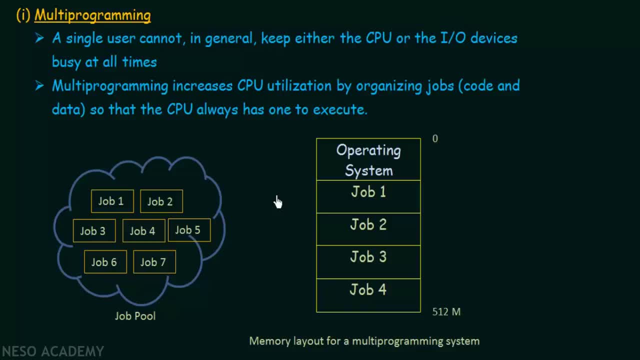 or when the lawyer is waiting for his paper works to be done. he does not simply keep waiting for that single client, but at that same time he can take care of another client that is under him. So in that way he is utilizing his time and resources efficiently. 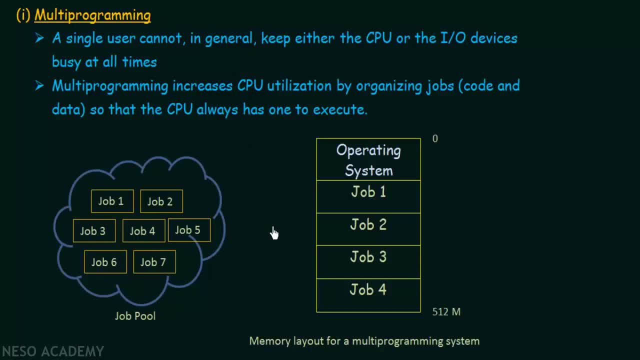 So that is what we do in multi-programming: We are trying to utilize our CPU efficiently. Now, a multi-programmed system provides an environment in which the various system resources, like CPU memory and peripheral devices, are used effectively, but they do not provide for user interaction with the computer system. 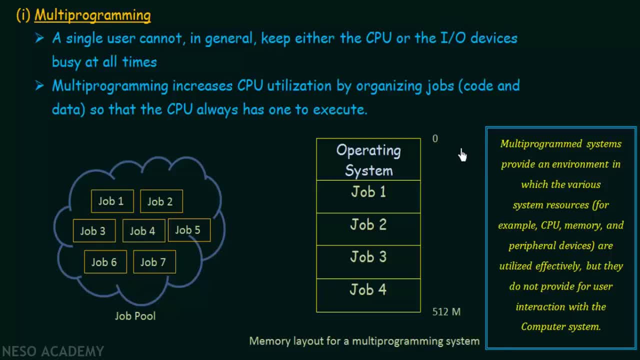 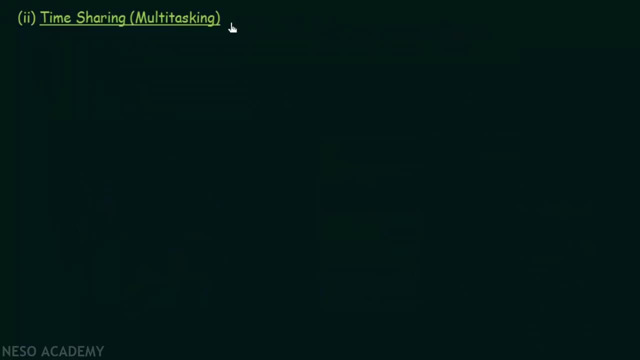 So in multi-programming system it makes sure that all our resources are used effectively, but they do not provide for user interaction with the computer system. So that brings us to the next topic, which is multitasking or time-sharing systems. So now let's see. what is this time-sharing or multi-tasking system? 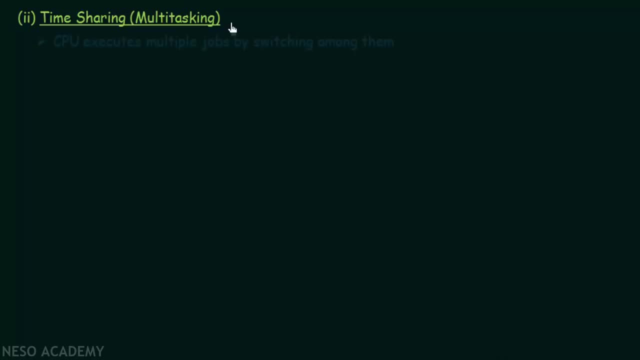 and let us see how it is different from the multi-programming system. So, first of all, the CPU executes multiple jobs by switching among them. Now, this is almost same like the multi-programming system. This first point: it says that the CPU executes multiple jobs. 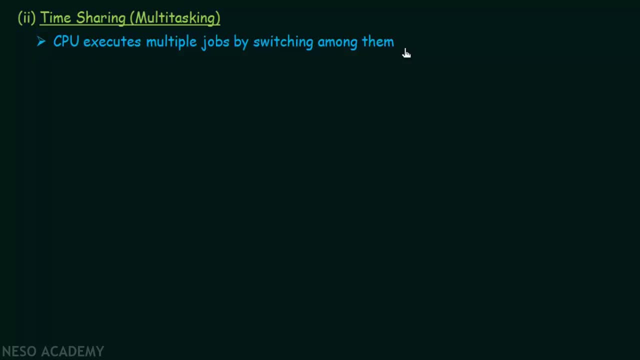 jobs. we have multiple jobs, as we saw above, and then, instead of executing only a single job at a time, what the CPU does is it switches between the jobs, and then the switching occurs so frequently that the user can interact with each program while it is running. now, when the switching happens, it happens so quickly. 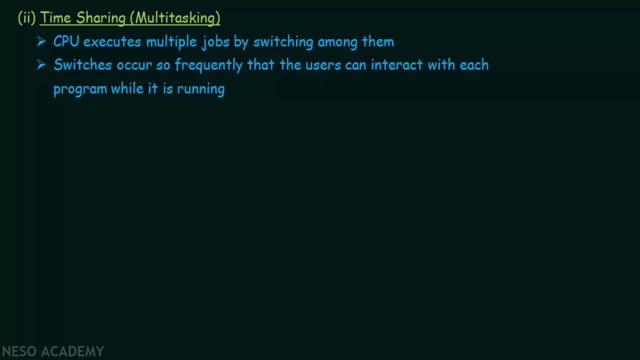 that the user can interact with the program while it is running. so this was something that was not there in the multi programming. so here the user can actually interact with the program even while it is running, because the switching between the jobs takes place very fast in this time sharing system. 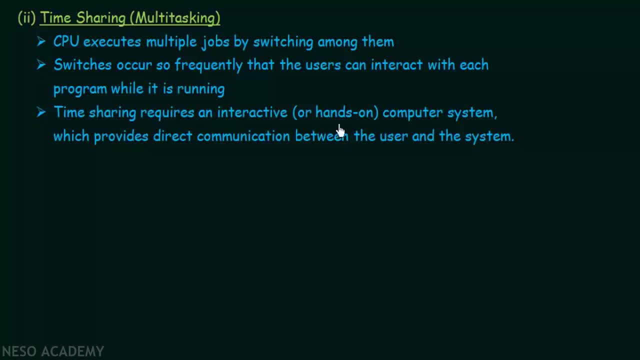 and then this time sharing requires an interactive or hands-on computer system which provides direct communication between the user and the system. so this was something that was not there in the multi programming system. there was a last point that we discussed, but in this time sharing system you can interact with the user and the system and the system is active and they. 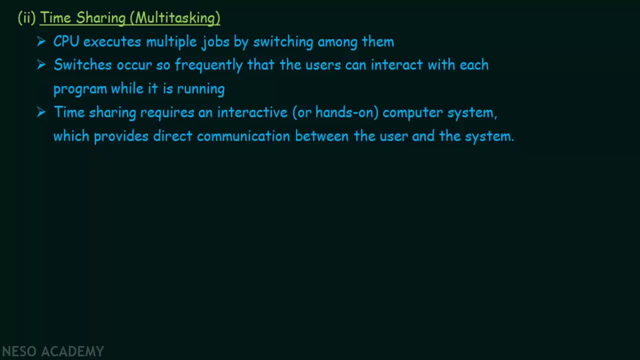 there is a direct communication between the user and the system And in this time sharing system. as the name suggests, a time shared operating system allows many users to share the computer simultaneously, So the computer system is shared among many users simultaneously in this time sharing system. 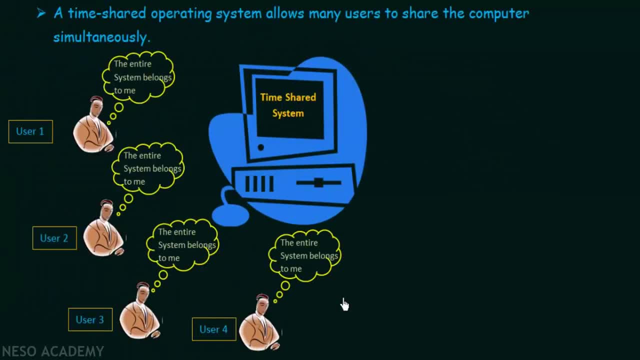 So let's see how this works. So, in order to elaborate this point, let us take an example. Let's say that we have a time shared system over here and there are four users sharing this system: User 1,, 2,, 3 and 4.. They are sharing this time shared system. Now, in this time sharing system, the switching between the jobs of the users takes place so quickly that the users themselves do not even realize that they are sharing the system. They feel that the entire system belongs to just that one person. So user 1,- he thinks that the entire system belongs to me, And user 2,, 3,, 4, all think the same, Because the switching between the jobs takes place so quickly that they don't even realize that there is a time sharing or multitasking happening in this system. 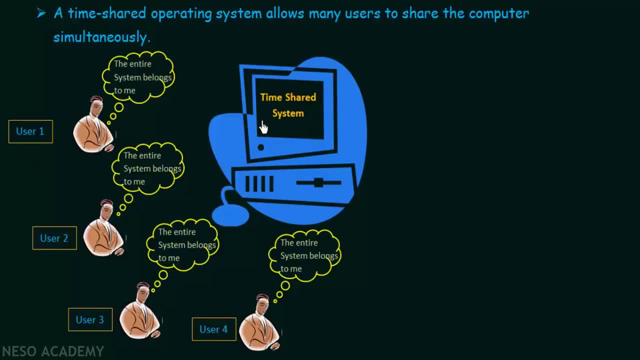 Now let's say that user 1 is using this time shared system and there is a certain job that he wants to execute. So the job is being executed by the time shared system and then the execution of the job takes place in CPU speed. 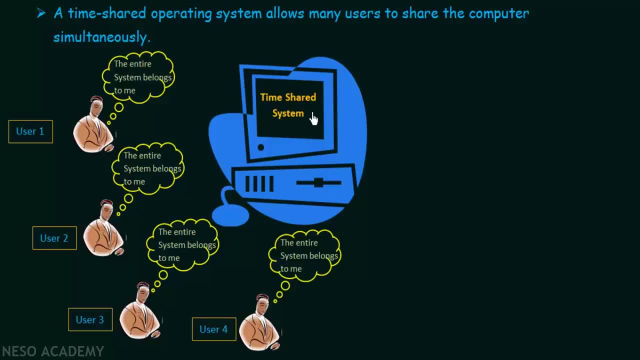 And we know that CPU speed is very high. So the execution of the job takes place in CPU speed And let's say that after execution the user has to be shown some output and then the user has to give some input again to the system. 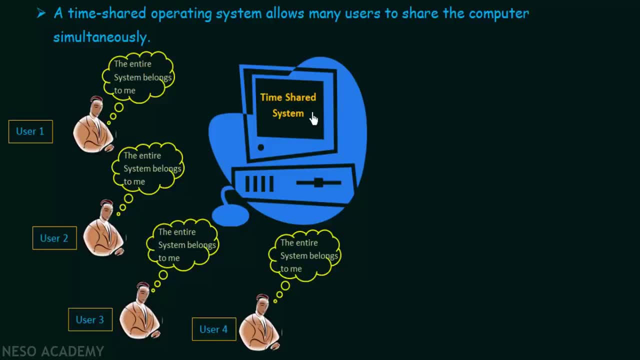 So after the execution of the job, the output is shown to this user 1 and user 1 wants to give some other input to the system. That means he is interacting with the system Now- the interaction between the user and the system. 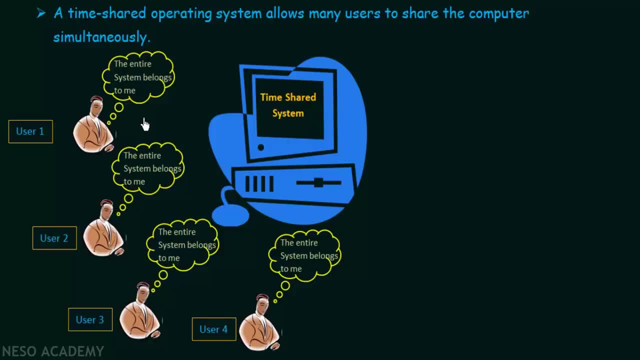 it takes place in user speed or people speed. That means it is taking place in human speed. So we know that CPU speed is so much higher as compared to human speed. So when he gives an input to the system, he is giving in the normal human speed. 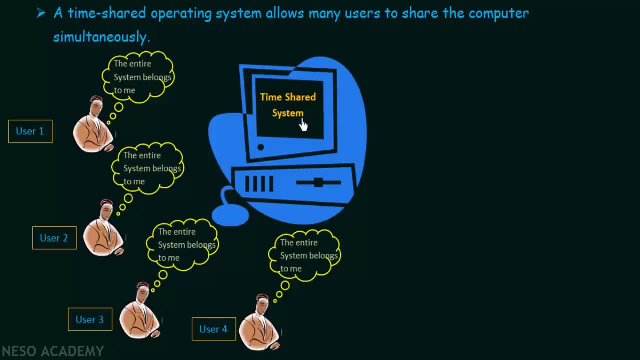 So that time gap itself is so big for the system that we have because systems are very fast. So while he is giving that input to the system in that time gap the CPU can be used by user 2 for executing the job from user 2.. 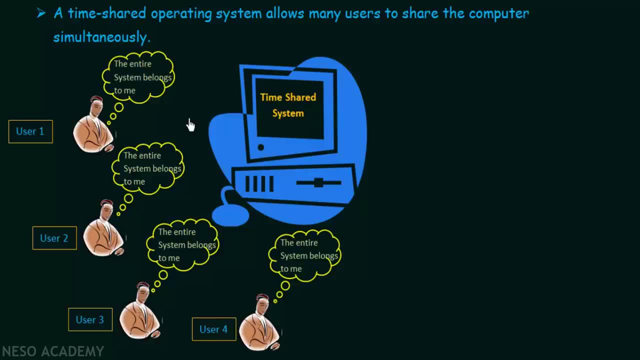 So in that way we see that there is a time gap between the user and the system, Because users are usually slower than the system. So in that time gap the switching of the jobs takes place so quickly and it is so quick and so frequent that 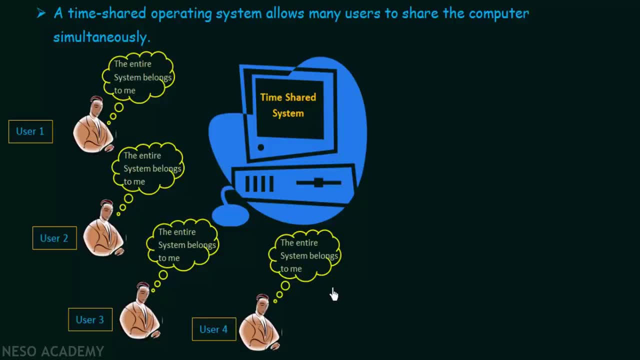 the user does not even realize that they are using a time-shared system. They just feel like the entire system belongs to themselves. So in this time-shared system it uses CPU scheduling and multi-programming to provide each user with a small portion of the time-shared computer.